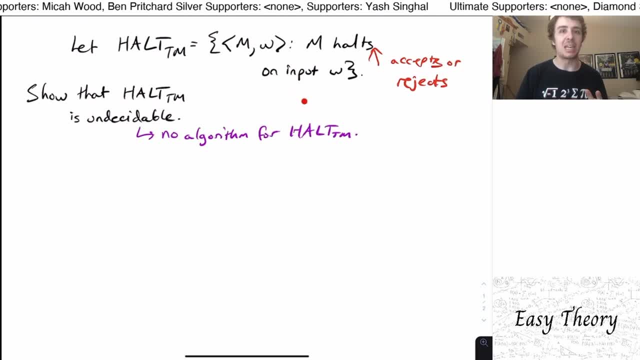 So you can show that it's undecidable by showing a known undecidable problem to be decidable under the assumption that this one is decidable. That's one route, and the other direction or the other possible route is to use Rice's theorem. But we can't use Rice's theorem here because that requires 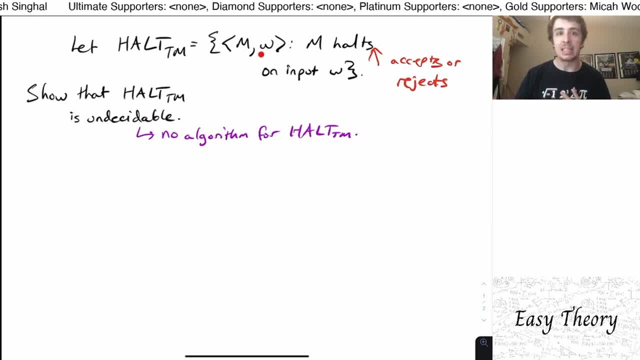 the strings in here to represent single machines and here they represent a machine and an input. So we can't use Rice's theorem here, unfortunately. So what we can do is to use a known, undecidable problem. So what we're going to use- assume- here- is: 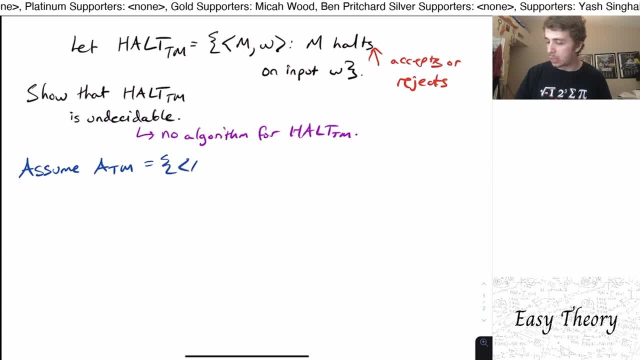 that ATM, which is the language MW, where M accepts W. we're going to assume that this is undecidable, because it is. And why do we want to use this language? Well, we got to use some undecidable problem first, and this one is undecidable because it's undecidable. So we're going to use MW where. 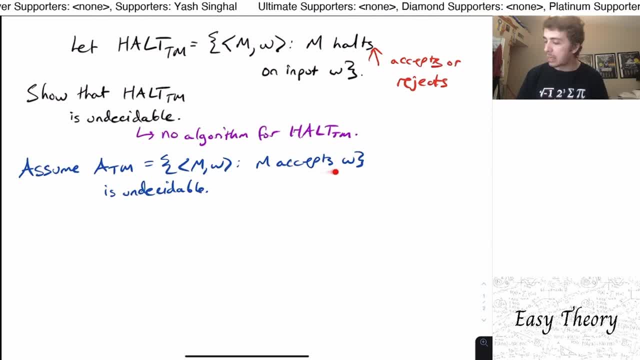 M accepts W and this one is a reasonable candidate to pick because the condition on whether MW is in this language or this one is very similar between the two. This one is it accepts W and this one is either halts an input W, either it accepts or rejects W. So here's what we're going to do here. 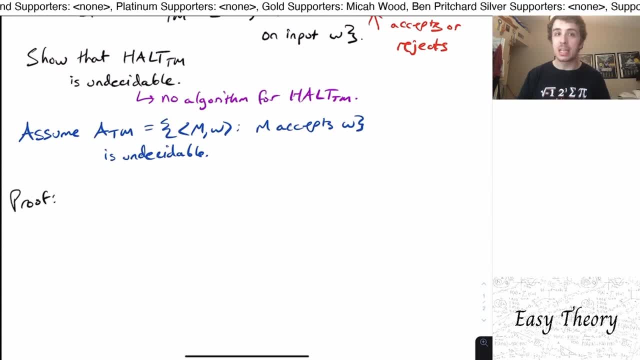 So how do we prove this, that halt TM is undecidable? Well, we want to assume that MW is undecidable. then, under that assumption, make a decider for ATM. So the problem with ATM and showing that it's decidable is the easiest way to do. it is just to run the machine M on W, but the Turing machine could. 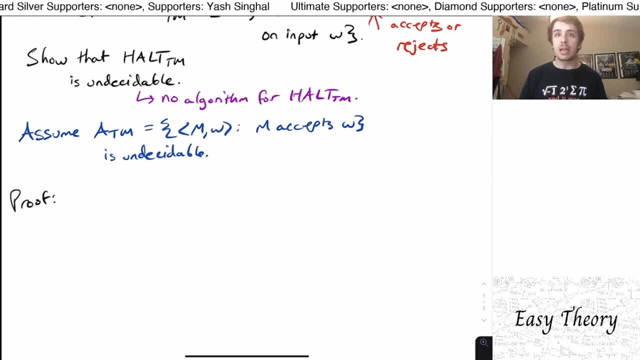 run forever. So what we can do here is if we had a way to figure out whether the machine halts on the input W to start with, then we can decide what actually happens. So what we're going to do here is on input W with M on W. So let's suppose that we're going to have a machine called H decides. 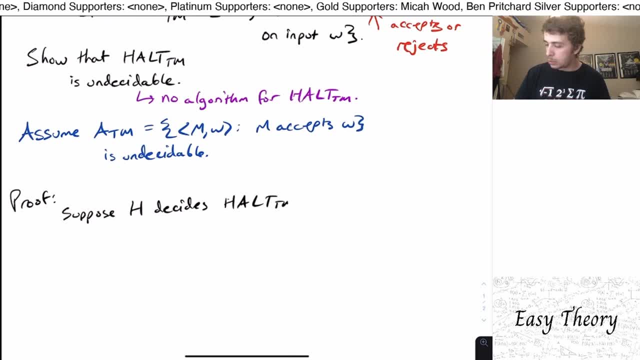 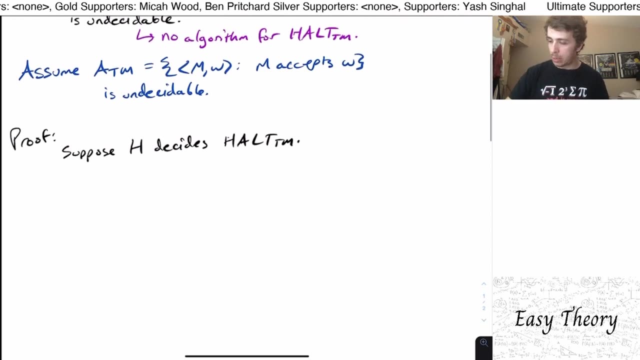 the language halt TM. So this machine H, if I give it an input M and W, I'm supposing that in some finite amount of time it'll tell me whether the Turing machine accepts the input or not. And so now let's build a decider for the language ATM. So remember, ATM must take input M W right here. So on input M W where? 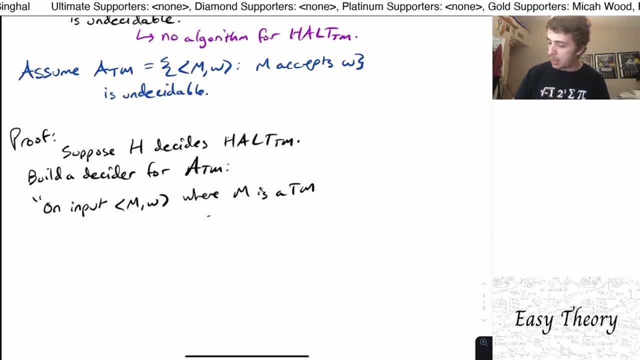 M is a Turing machine and W a string. Well, if I just try to run the machine M on W again, it could run forever. So let's utilize this decider H to figure out whether the machine even stops or not. So let's run H on M, W. Well, H will either say it does halt. 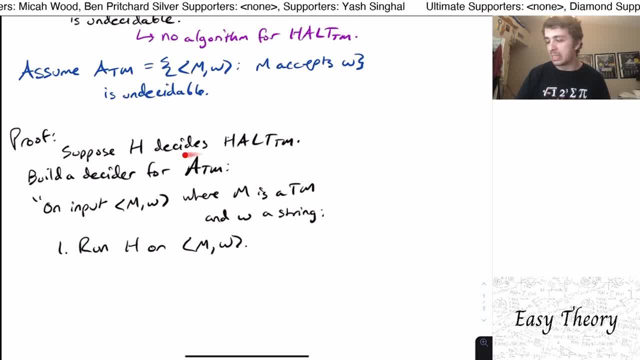 or it doesn't, because we're supposing that it decides. this machine decides that language. So let's suppose that H rejects. So if H rejects, then that says that M does not will run forever on input W, which implicitly says that the machine will implicitly reject W just by running forever. It never accepts W. So for the 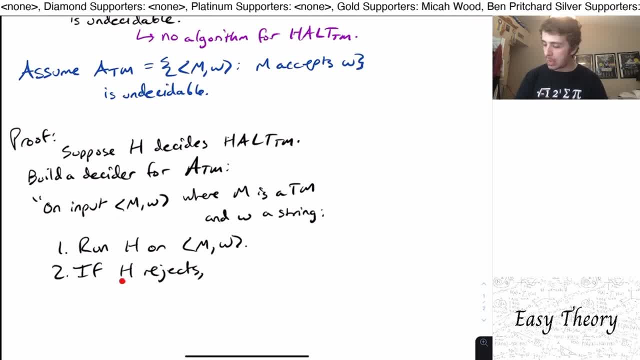 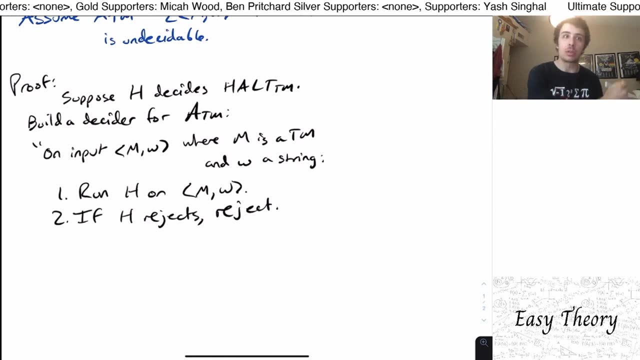 question of whether M accepts W. if H rejects, M does not stop on input W, so it never accepts in that case. So here we can actually say reject Because, um, we want to say accept only when M actually explicitly accepts W In every other case. 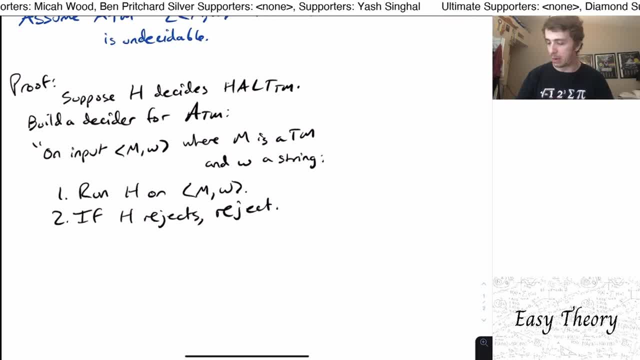 it. just we should say: reject, even if it runs forever. So then here, if H doesn't reject, in which means that it accepts, which this implies that M does stop on W, it doesn't run forever. So what we can say here is that M 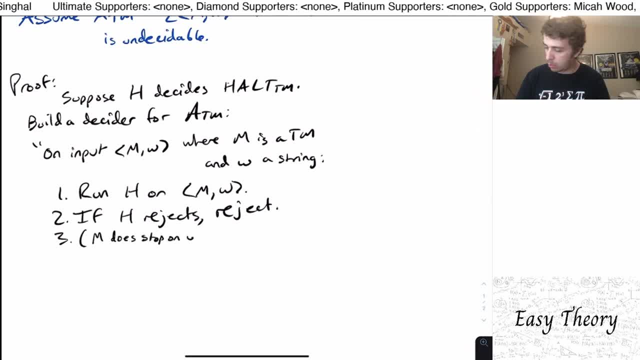 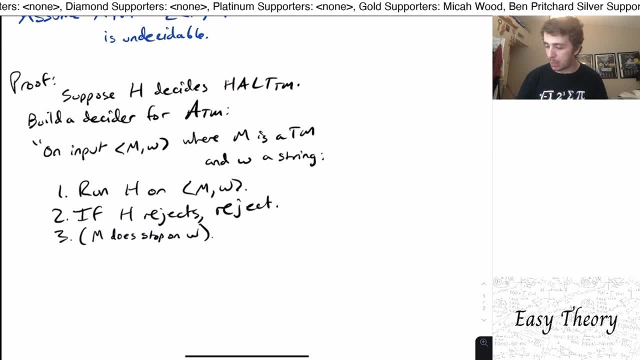 does stop on w. well, now we can be certain that it stops on w. so now we can actually run the machine on input w. so let's actually run m on w this time. so just run the machine because we know that it will stop here, based on the assumption that h will reject before. so if we 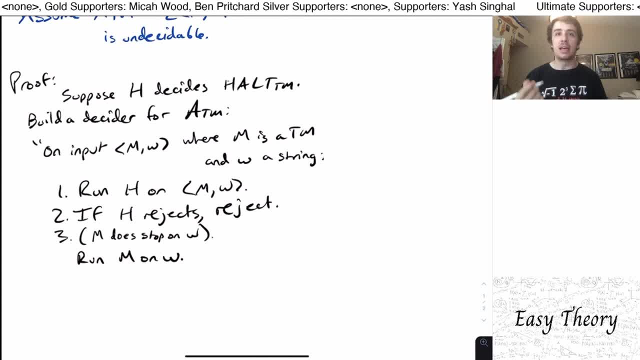 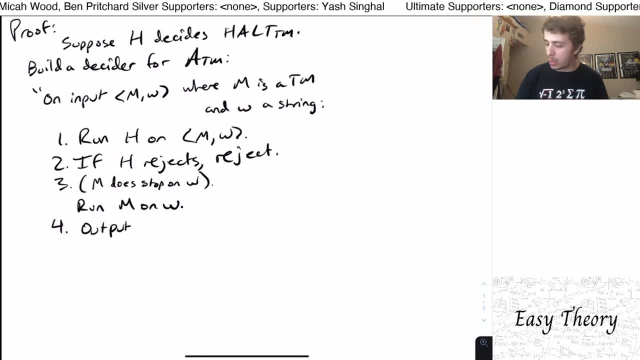 make it to this step. that means h said that the machine will stop on the on w. so then now all that we need to do is to output the same answer. so whatever m says on w, we're gonna do the exact same thing. if m accepts w, then we're gonna say accept. if m just plain outright rejects w, then 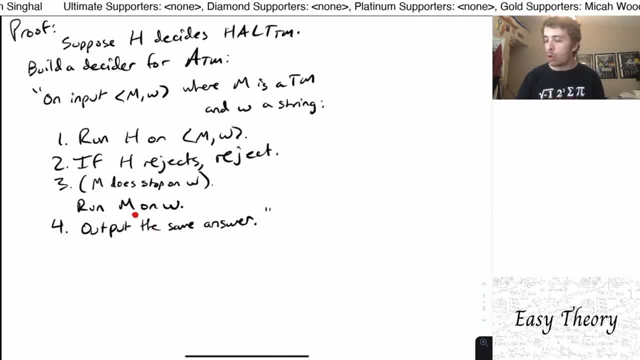 we'll just reject in the exact same way, and we know, if we make it to this step, that h said that the machine will stop on w, so now all that we need to do is to output the same answer. so it to step 3. one of those two will happen, because we saw that H told us. if 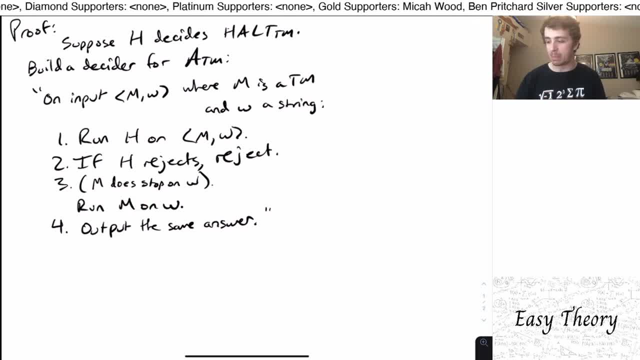 we get to this step, if the machine will stop on input W. well, now let's actually figure out whether we can even build this machine. well, we can do step 1 based on the supposition. so the supposition here told us that H exists. it's a. 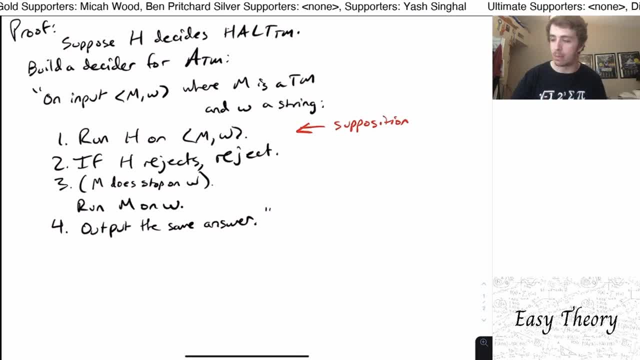 decider for halt TM, so we can actually do this step in a finite amount of time. well, these two steps run in a finite amount of time because, well, step 2 is pretty clearly going to run in a finite amount of time step 3 does, because H. 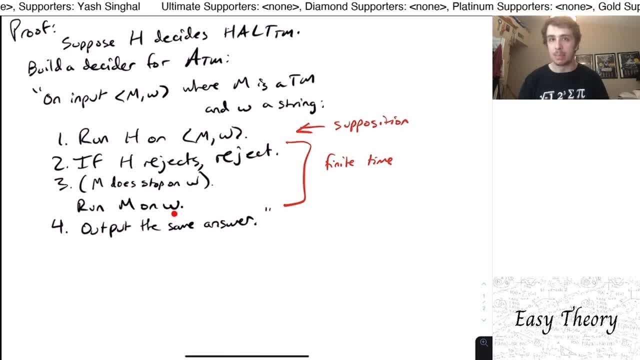 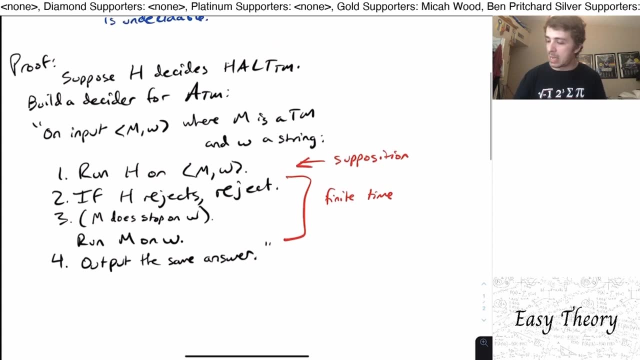 guarantees that M will stop on input W. it can't run forever, because if it did we would have stopped in step 2 above. and then step 4 obviously runs in a finite amount of time too, so that would imply that ATM is decidable. you can't run in a finite amount of time because if H is decidable, then we can. 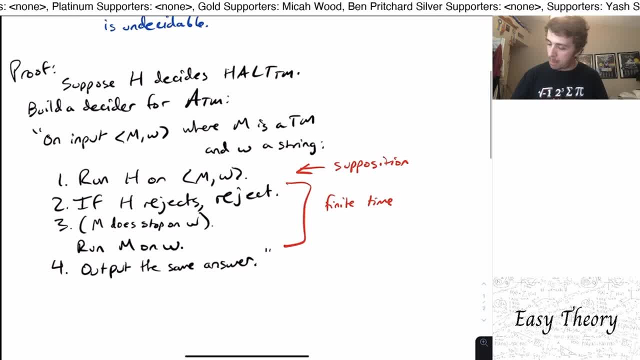 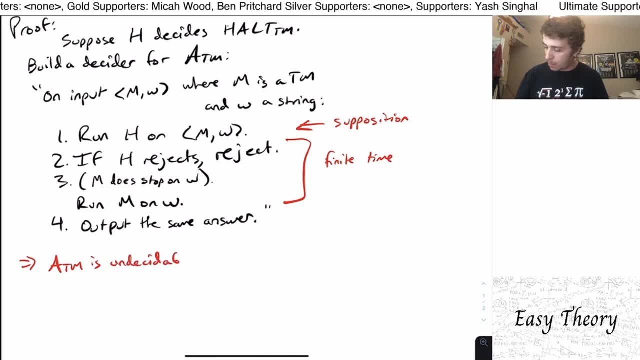 build this machine that runs in a finite amount of time, which implies that ATM is decidable. but we know that ATM is undecidable, so this implies that the decider H here cannot exist, because if it did, then we could build this machine, which is a contradiction. so this means that H